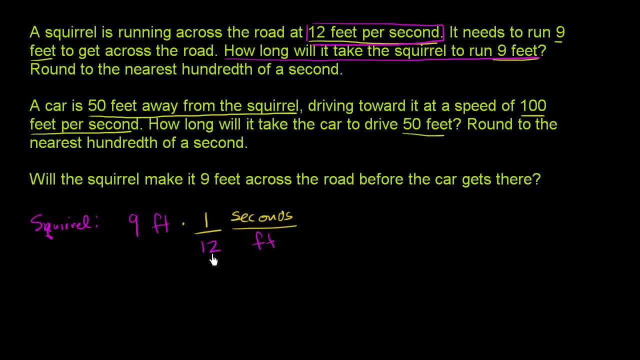 12 feet per second and I wrote it as second per foot. 12 feet for every 1 second. 1 second for every 12 feet. What's useful about this is this will now give me the time it takes for the squirrel in seconds. 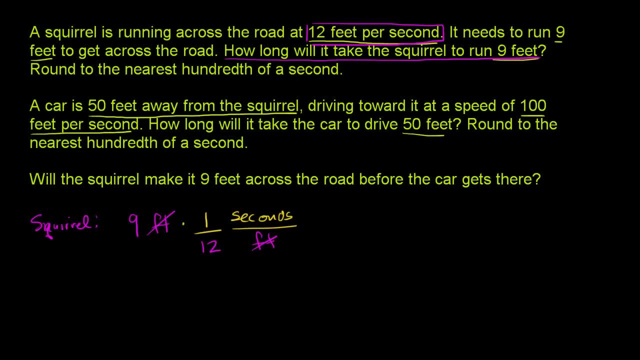 So the feet cancel out with the feet and I am left with 9 times 1 12th, which is 9 12th seconds, And 9 12th seconds is the same thing as 3 4th seconds. 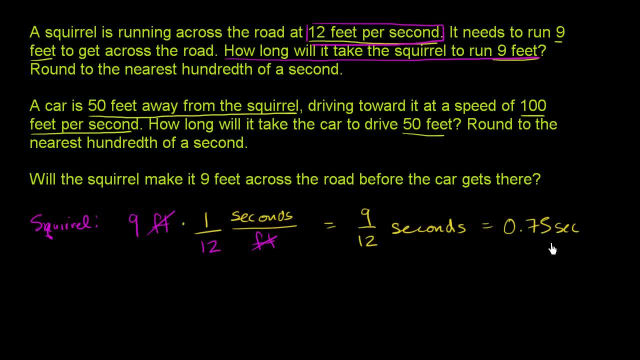 which is the same thing as 0.75 seconds for the squirrel to cross The street. Now let's think about the car. So now let's think about the car, And it's the exact same logic. They tell us that the car is 50 feet away. 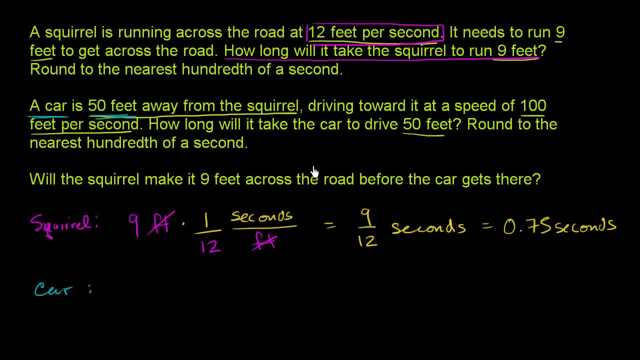 So the squirrel is trying to cross the road like that And the car is 50 feet away, coming in like that And we want to figure out if the squirrel will survive. So the car is 50 feet away, So it's 50 feet away. 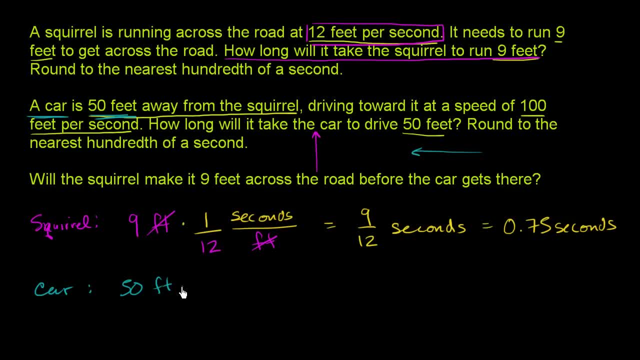 We want to figure out the time it'll take to travel that 50 feet. Once again, we would want it in seconds, So we would want seconds per feet, So we would want to multiply by seconds per foot. They give us the speed in feet per second. 100 feet per second. 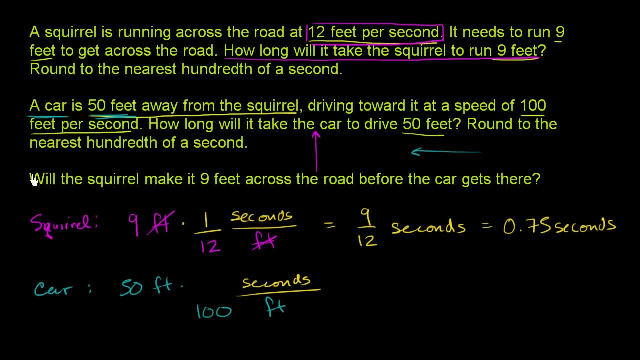 And so we just have to realize that this is 100 feet for every 1 second, or 1 100th seconds per feet. This is, once again, just this information, this information, But we took, We took the reciprocal of it. 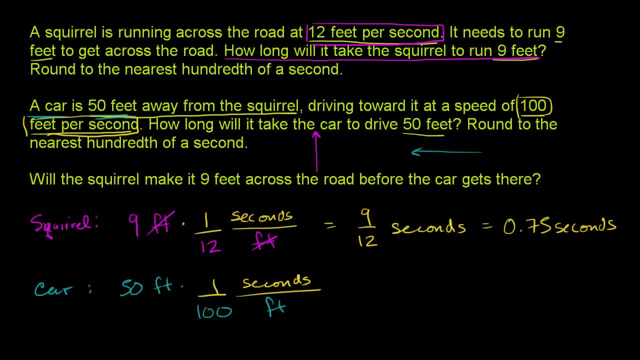 Because we don't want feet per second, We want seconds per feet, And if we do that, that cancels with that And we're left with 50 over 100 seconds. So this is 50 over 100 is 0.50 seconds. 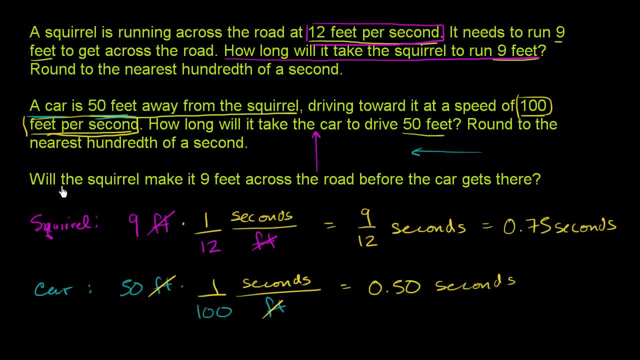 And so now let's answer the question: this life and death situation for the squirrel. Will the squirrel make it 9 feet across the road before the car gets there? Well, it's going to take the squirrel 0.75 seconds to cross, and it's going to take the car only half a second.